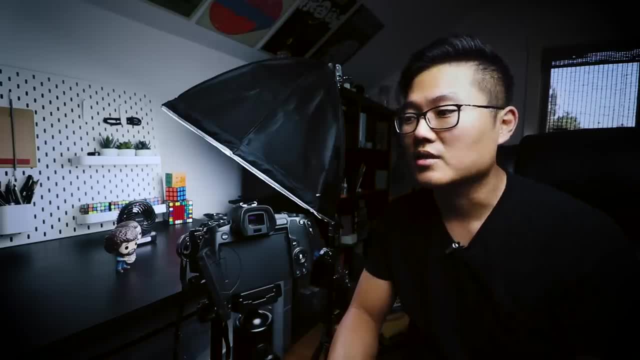 So today we're going to talk about how to shoot manual, and this is probably one of the most popular topics for beginners, and you might be here because you just bought yourself your first camera, or maybe you've been doing photography for a while, but you want to take your photography to the next. 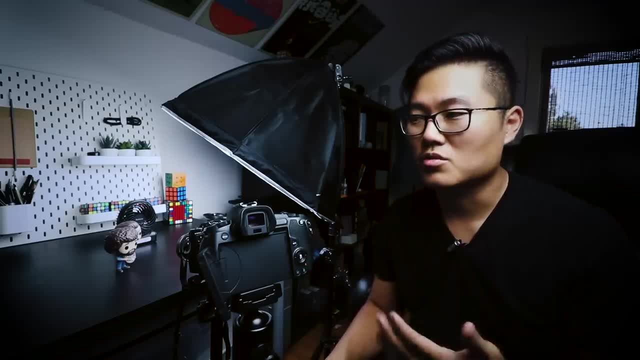 level and you've been probably hearing from people all the time that you should shoot in manual. but you know, don't get me wrong- I'm not one of those people who says that you're not a real photographer if you don't shoot in manual. I personally don't care what other people do, but you have to understand. 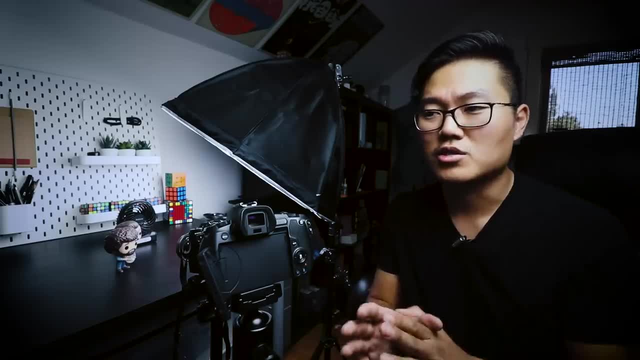 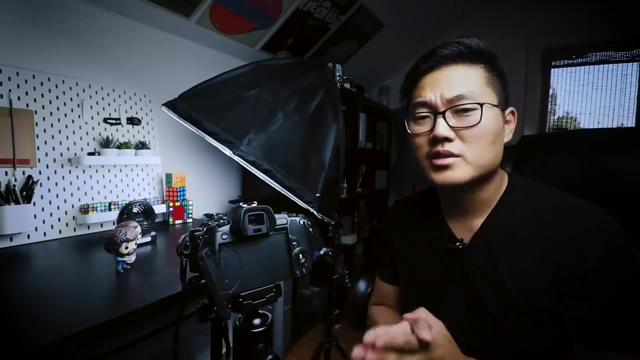 that there's a big difference between not shooting manual because you don't know how and why and not shooting manual because it may not really affect your photography very much. So you have to understand that there is a difference. and if you're not shooting manual because you don't know how, then 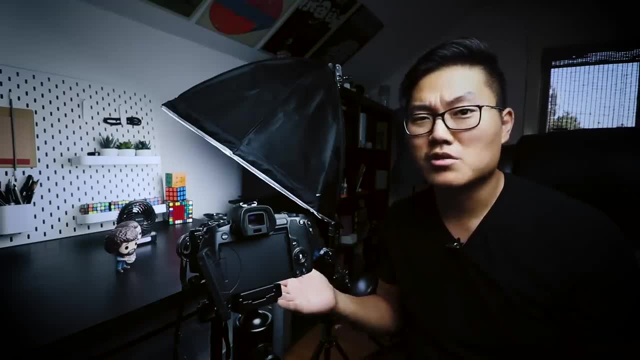 you're really not going to go far as a photographer. So, and there's no reason not to learn because it's so easy, and just by watching this video and some practice, you should be able to shoot in full manual in no time, I promise. So let's get started. Okay, so I'm filming the back of my camera pointed at a. 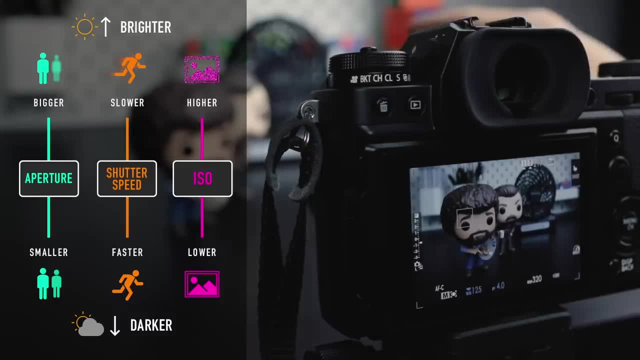 few shots. So I'm going to start with the back of my camera pointed at a few shots. So I'm going to things on my desk and please excuse me for the noise of the fan back there. that's there for a reason and on the left side of your screen I made this. 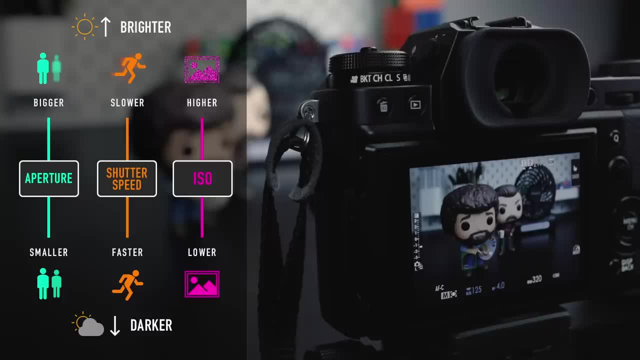 simple graphic so it's easier for you guys to see what I'm doing. so, when it comes to shooting manual, there are three things you have to remember: aperture, shutter speed and ISO. these are the three things that you're gonna be constantly adjusting on your camera when you're shooting in manual, and I know 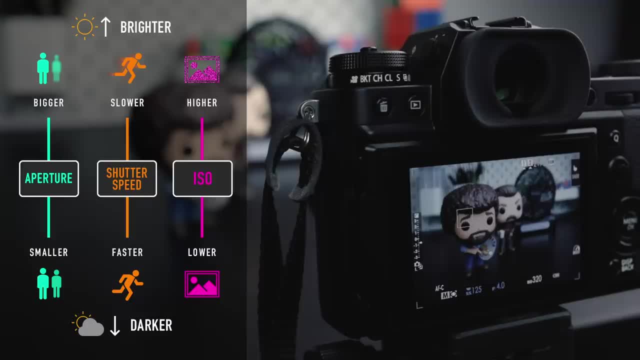 that may sound a little complicated right now, but once you understand what they are and learn how they work together, it'll be a lot easier to understand, I promise you. so the first thing is aperture. aperture actually has more to do with the lens than your camera itself, and when the aperture is 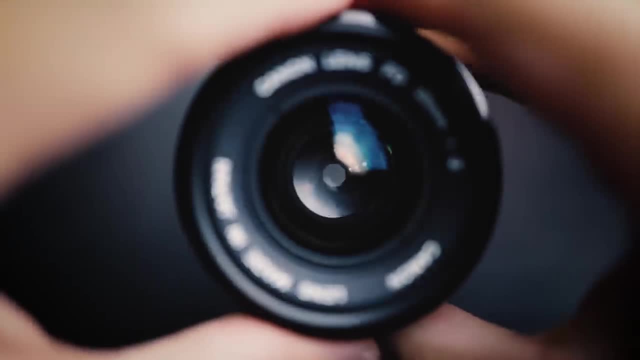 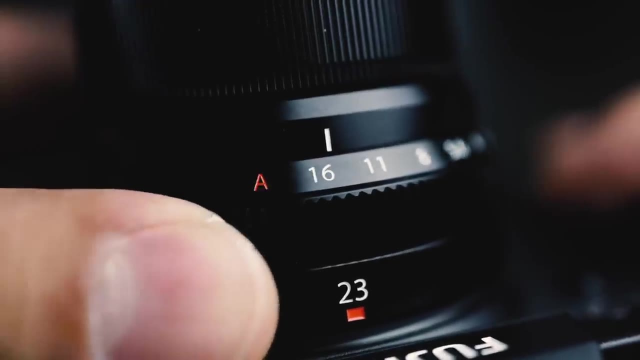 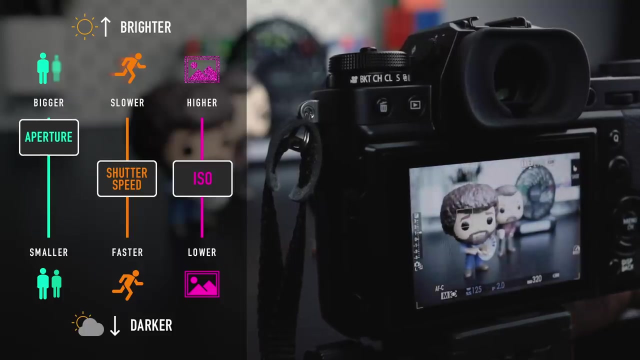 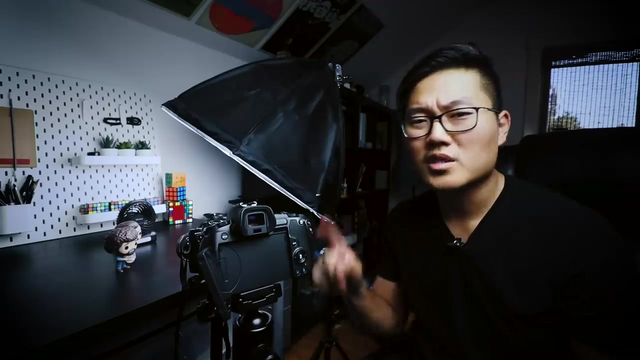 wide open your lens lets in more light into your camera, therefore making your images brighter. so bigger aperture, more light, smaller aperture, less light. pretty easy to understand, right? so let me demonstrate right now. I'm going to increase my aperture all the way up to F 2 and, as you can see, the image gets a lot brighter. one thing that's kind of 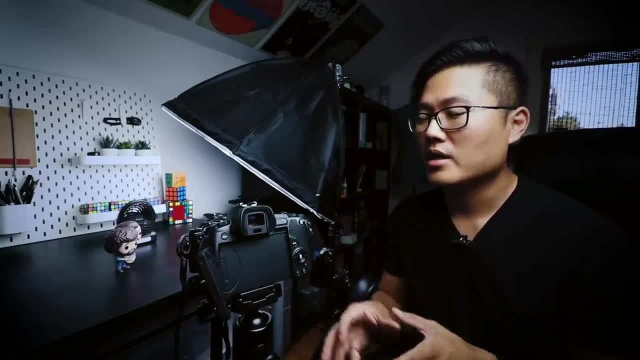 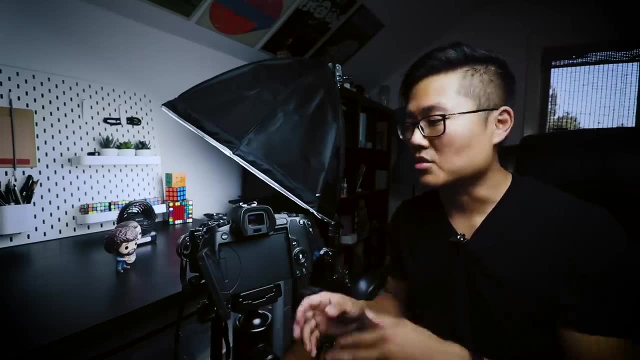 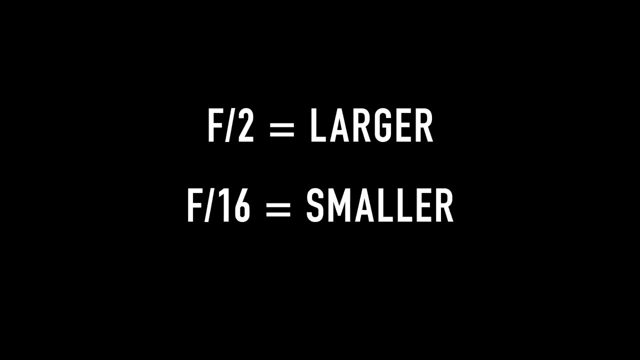 tricky that you have to remember is that the f-stop number and the size of the aperture that it represents are backwards. so the smaller the f-stop number means bigger the aperture. so, for example, on this particular lens, F 2 means bigger than F 16. you know at least. it's not some weird mathematical formula. 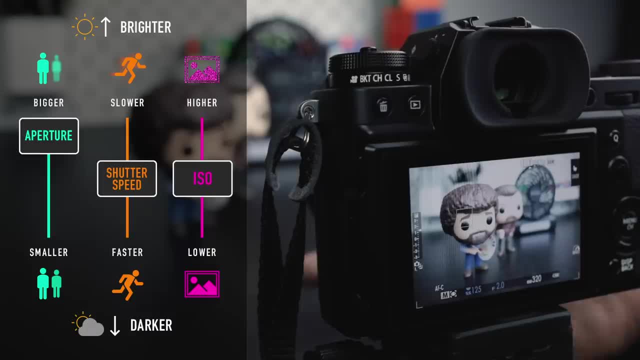 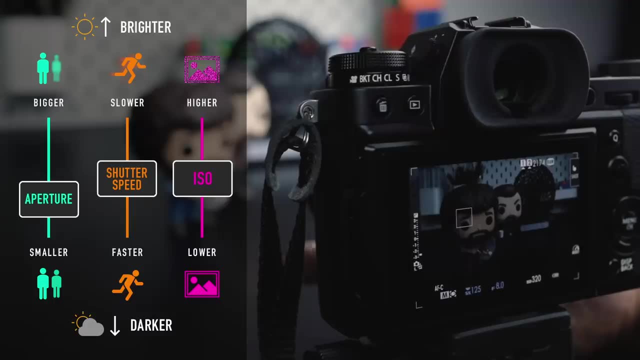 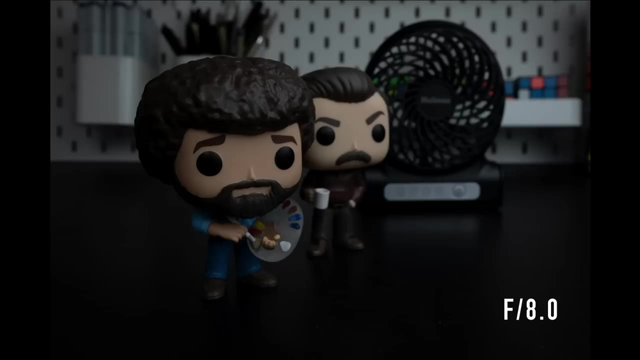 that you have to remember. you just have to know that it's the opposite. okay, and now I'm going to decrease the size of the aperture by increasing the f-stop number and all the way up to maybe F 8, and I'm going to take another photo and, as you can see, the image became a lot darker. so, again, 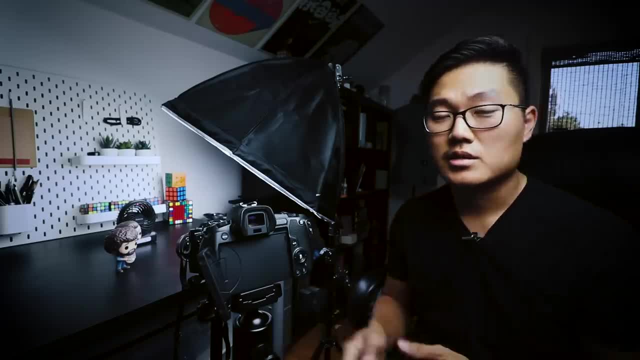 bigger aperture, more light. smaller aperture, less light. now let's move on to the shutter speed. shutter speed is what determines the amount of time that your sensor gets exposed at the shutter rate, and you can see that it's kind of like a movement like you would see on a shutter speed. so you can see that the shutter 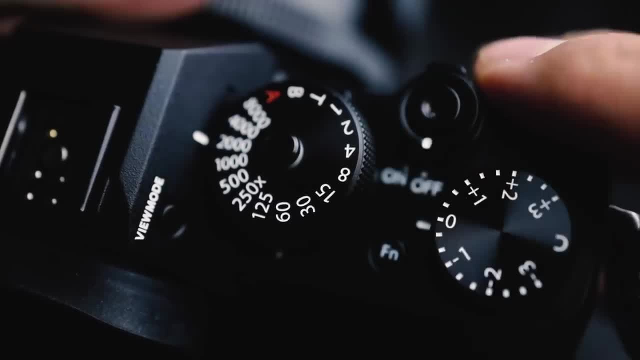 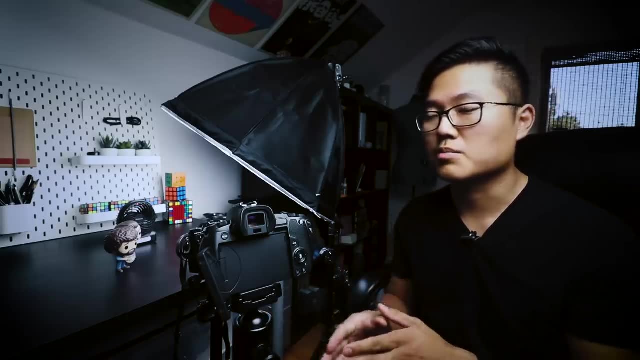 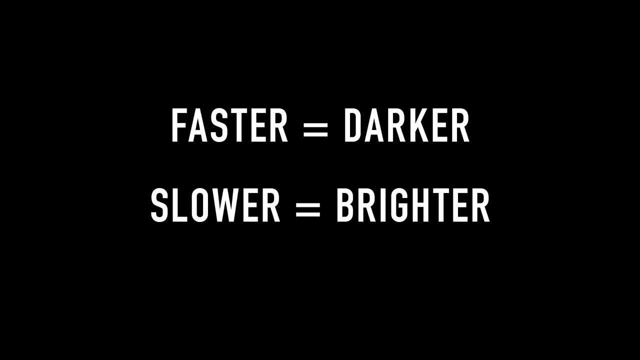 to the scenery or the light. So faster shutter speed means your sensor will get exposed to the light for a shorter amount of time. and slower shutter speed means your sensor will get exposed for a longer period of time. So faster shutter speed- darker. Slower shutter speed: brighter. Let me show you how that works. 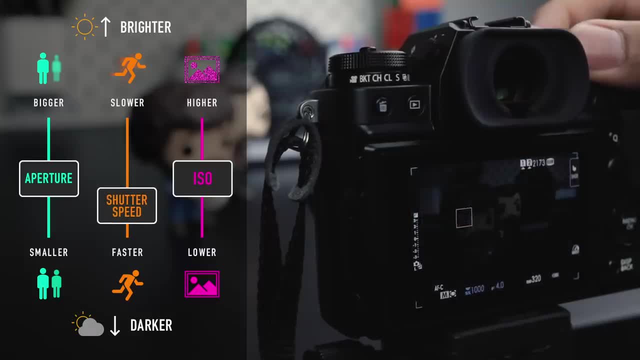 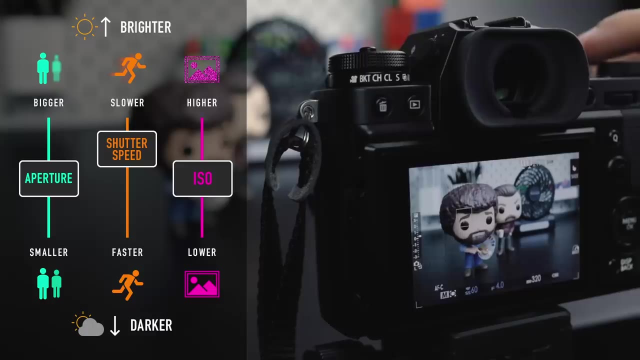 So now I'm going to increase my shutter speed and, as you can see, the image became a lot darker. I'm gonna take a photo here and then I'm going to slow down my shutter speed just about there and take another photo. So that's pretty. 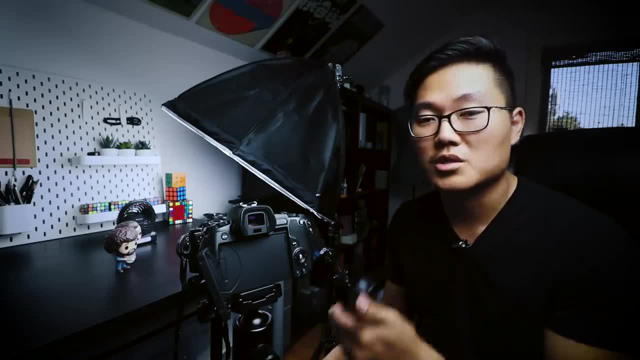 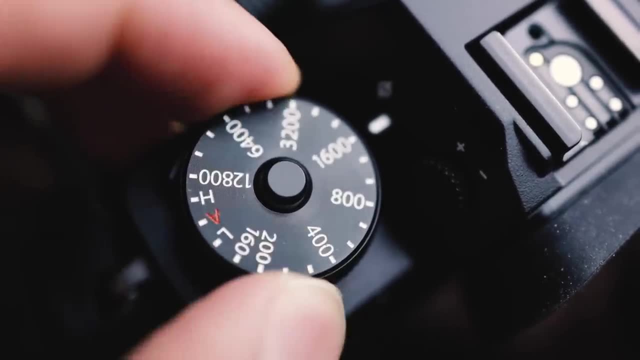 obvious, right? So that's how you change the brightness of your photo with your shutter speed. So now let's move on to ISO. ISO, you know. the name of it may not be as obvious as aperture or shutter speed, but in some ways you could think. 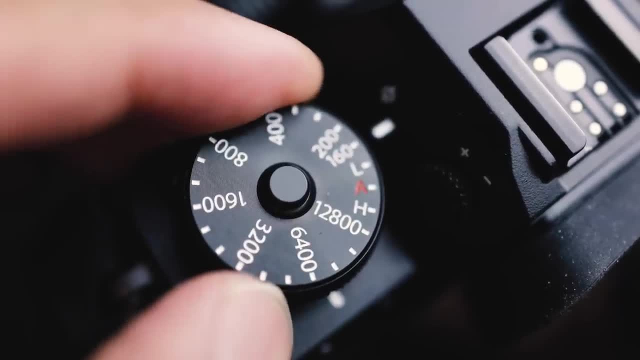 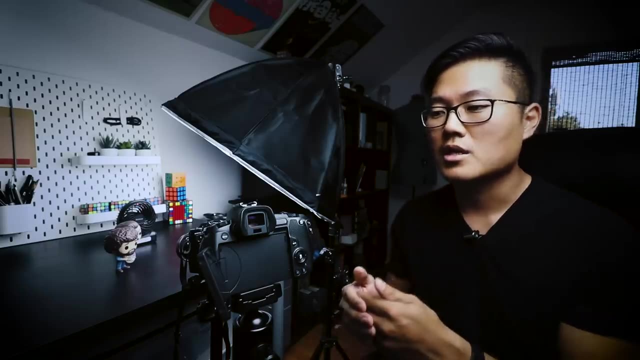 of it as like a volume knob on your stereo or microphone. So what the ISO does? it changes your shutter speed. So what the ISO does? it changes your camera's sensitivity to light. So when you increase the ISO, your camera becomes more sensitive to light. Therefore, your images become brighter. and when you 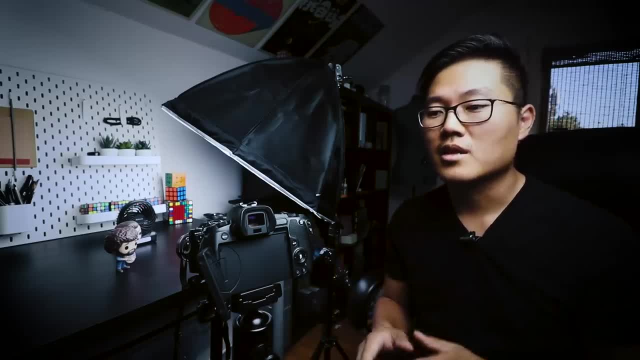 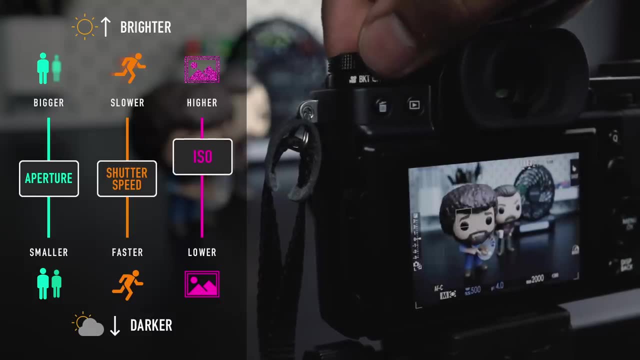 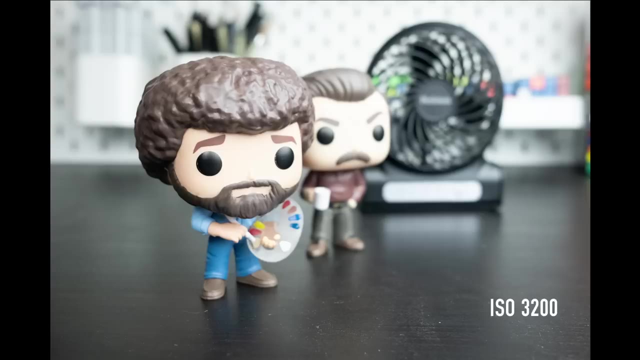 decrease the ISO on your camera, your camera becomes less sensitive to light, Therefore making your images darker. Let me demonstrate. So first I'm going to increase the ISO all the way up to ISO 3200 and then take a picture. and then I'm going to decrease the ISO all the way up to ISO 3200 and then take a picture, and 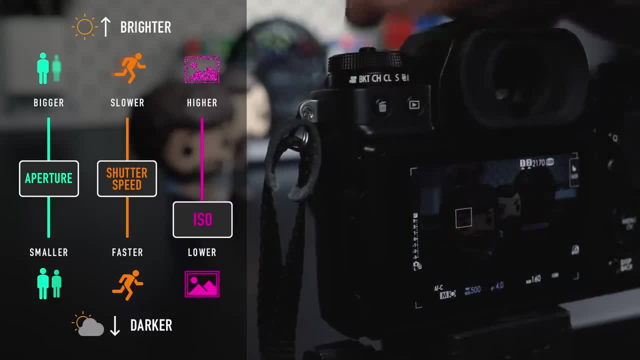 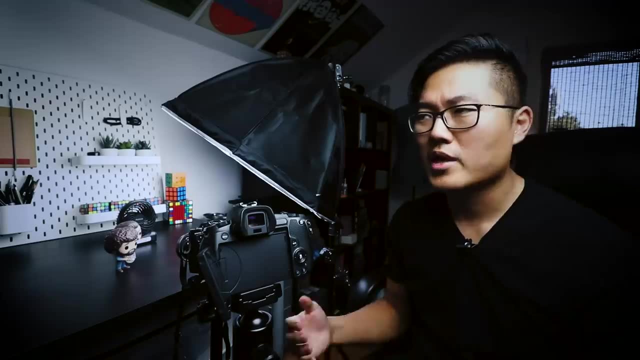 the ISO all the way back down to ISO 160 and again. clearly you can see the difference. so by now some of you might be thinking: so why do we need three different things to change the brightness? why don't we have just one big dial that says brightness? well, that is because all these three things have 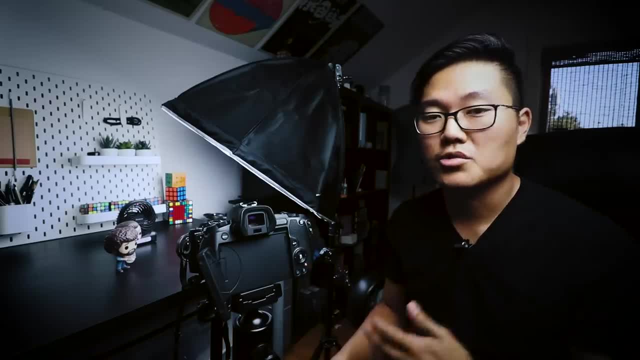 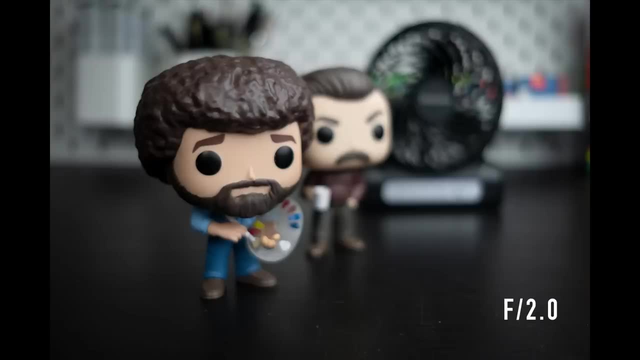 different side effects, and some of you might have already noticed when I showed you the side-by-side comparison, but let me demonstrate again. so right now I'm at f2, which is the widest aperture that this lens allows, and Bob Ross is in focus, but everything else seemed blurry, and that is because, with bigger aperture, 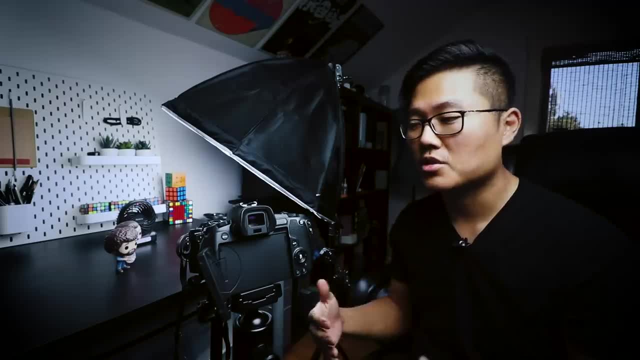 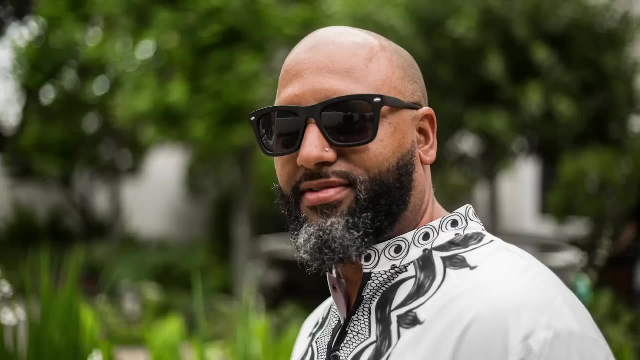 you get shallower depth of field, which means with a bigger aperture, the plane of view that's in focus will be shallower. so obviously this is useful when you're taking a portrait of someone with a nice blurry background. but what about when you want to take a family portrait or a group portrait with? 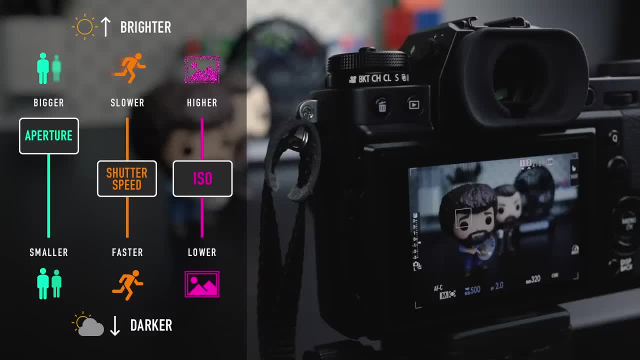 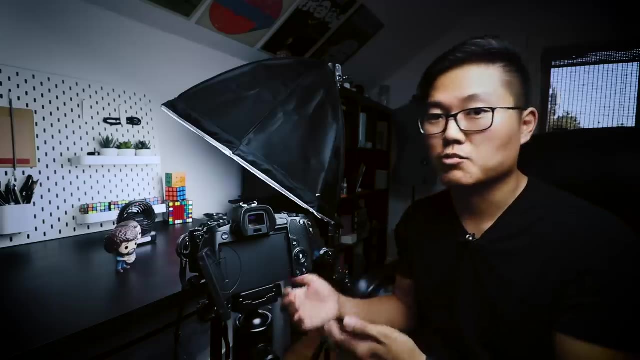 multiple people, in this case Bob Ross and Ron Swanson. what do you do when you want both of them to be the same? what you do is you decrease the size of your aperture- let's bring it down to maybe 5.6- and, as you can see, both of them are in focus now because 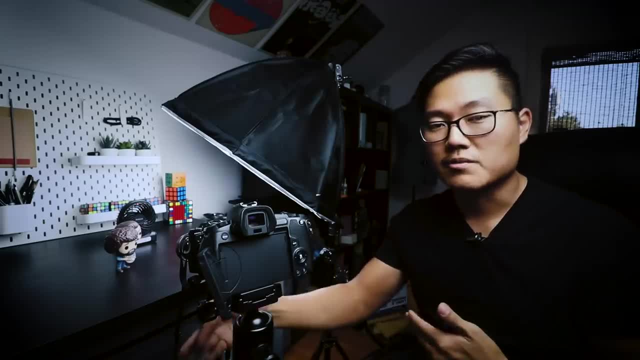 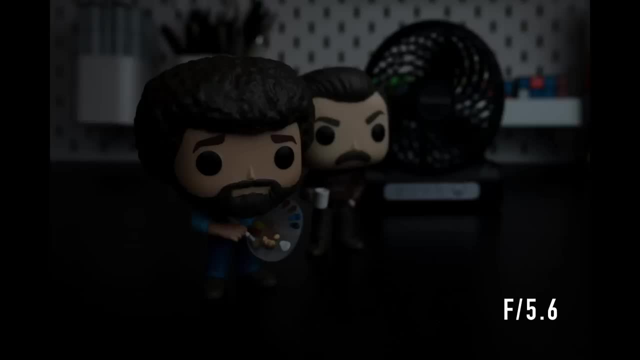 with smaller aperture again, you get deeper depth of field. so here's where it gets really interesting. so now both Bob Ross and Ron Swanson are in focus, but because of the small aperture your image is too dark. everything is underexposed. so what do you do? 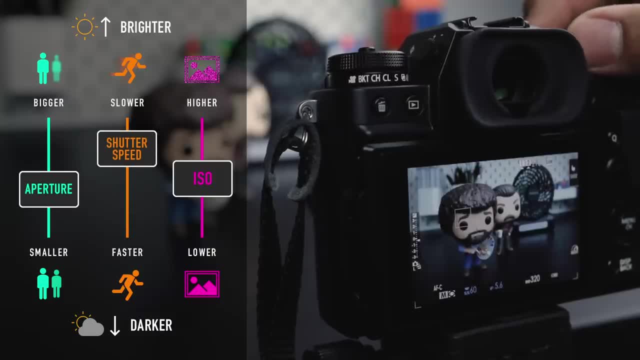 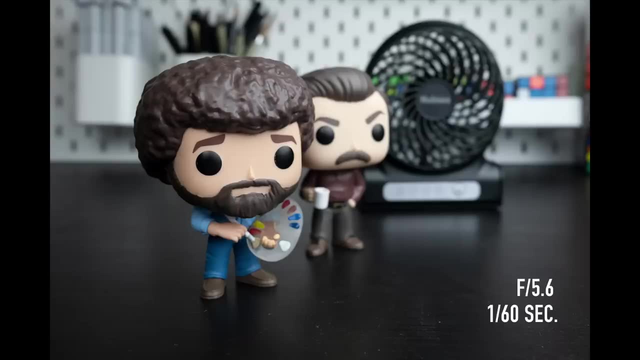 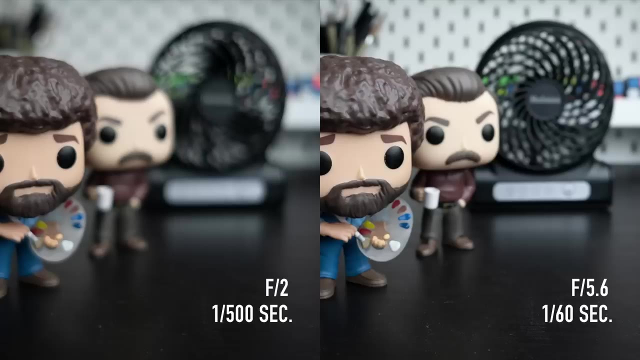 you can decrease the shutter speed and make the image bright again, and now both Bob Ross and Ron Swanson are in focus and everything is correctly exposed. but shutter speed also has its own side effect, and if you take a look at the fan in the back on the photo that was taken with the faster shutter speed it looks. 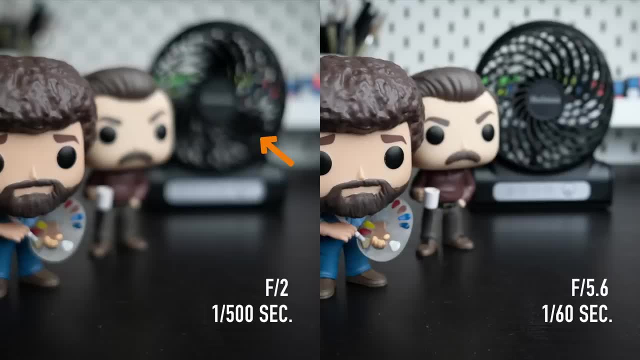 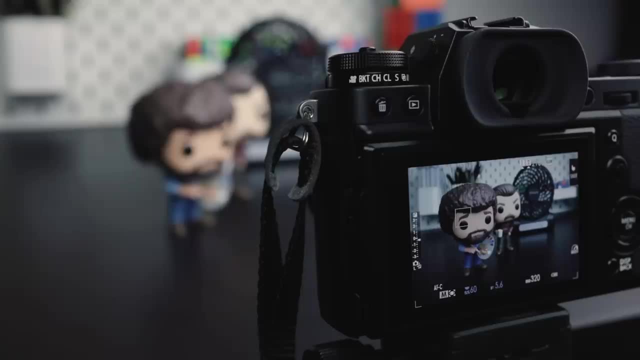 like the fan is barely spinning, but on the photo that was taken with a slower shutter speed, it looks like the fan is spinning so fast it's almost invisible. the fans been running at the same speed the entire time I'm recording this and this is all happening because of the shutter speed. so let's say you're taking 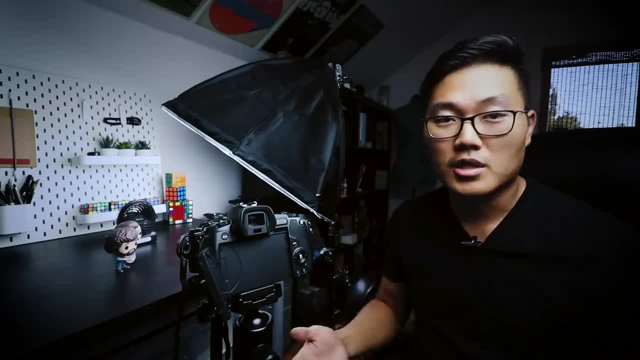 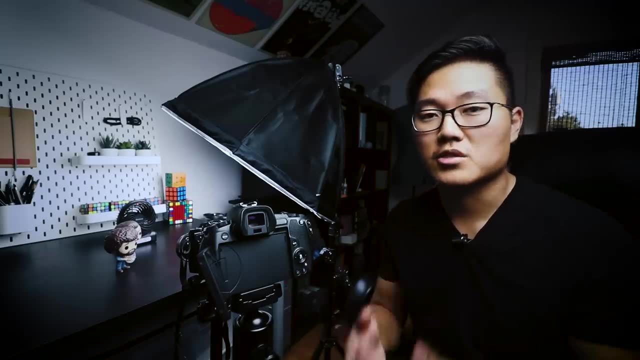 a family portrait and there's a bunch of children and, as we all know, children are biologically incapable of staying still. so you want to use smaller aperture because you want everyone's faces to be in focus. but then now you have to slow down your shutter speed because your image is underexposed. so imagine that. 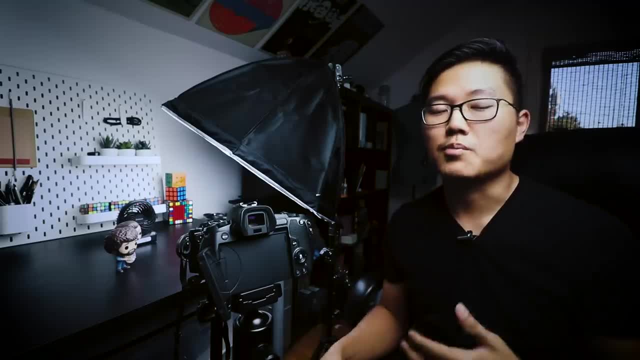 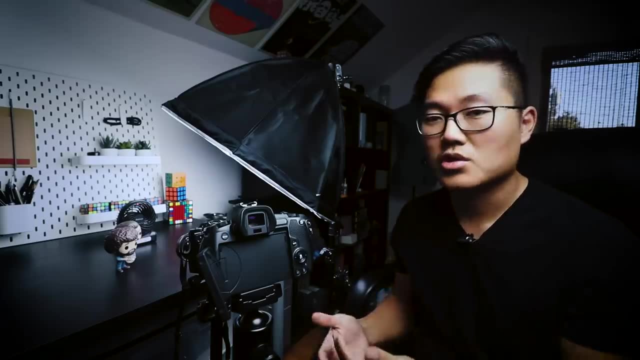 fan is like any sort of moving objects that you want to take a picture of. it could be some wild animals or wild animals animal. It could be your children. So, in order to prevent any sort of motion blur, you have to keep your shutter speed reasonably high whenever you're taking a photo- And it's not always the subjects. 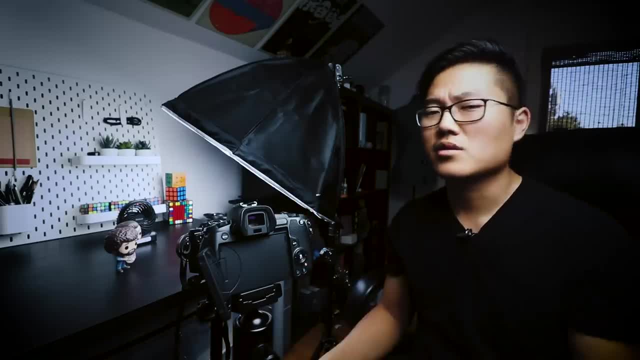 that move Your hands move as well, because you're alive. And I get a lot of comments from people saying that their photos are not sharp and they're asking me if they should get a new camera or a lens. But there's a very, very good chance that your shutter speed may not be high enough, So try. 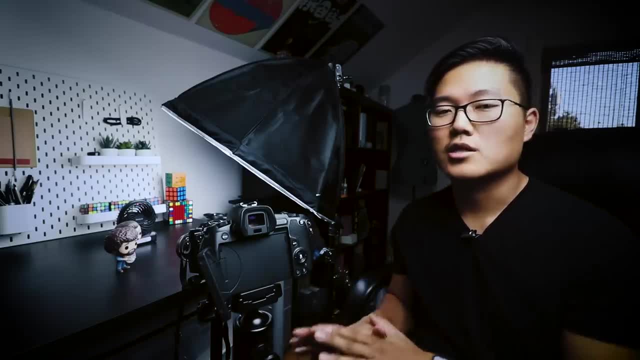 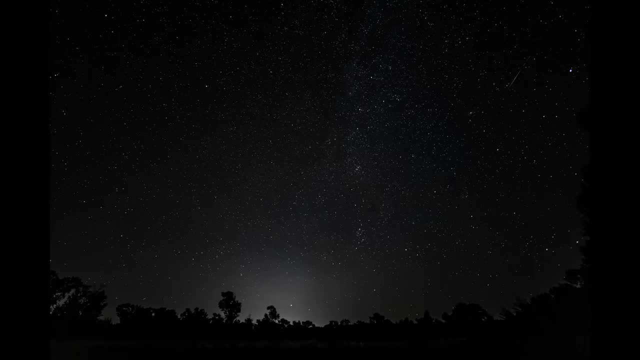 that first, And that doesn't mean that slower shutter speed is always bad. Sometimes you want that slower shutter speed to get certain effects or get long exposure, Like when you're doing night photography or light trail shots, or when you want to portray a certain motion of a musician or a 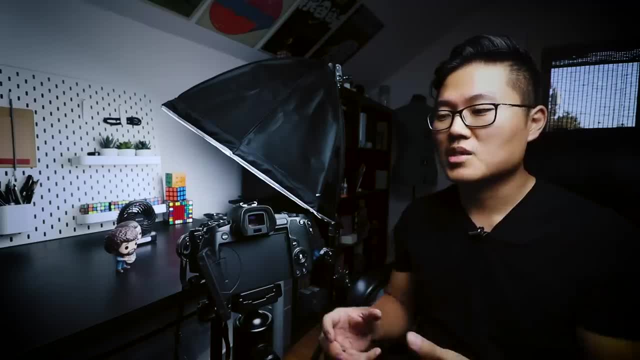 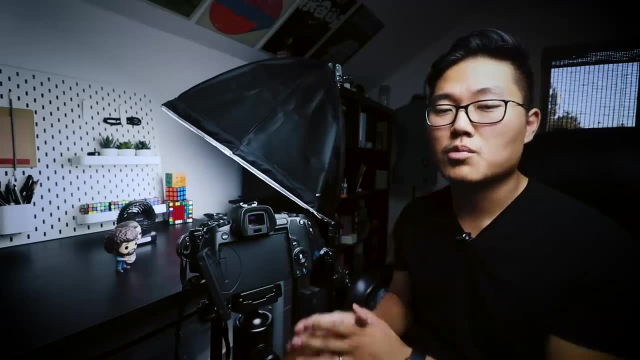 dancer. you can do a lot of cool things with slow shutter speed. You just have to keep your camera incredibly still or use a tripod. So let's say you're taking a group portrait and there's a bunch of children. You want to keep your aperture small so that everyone's 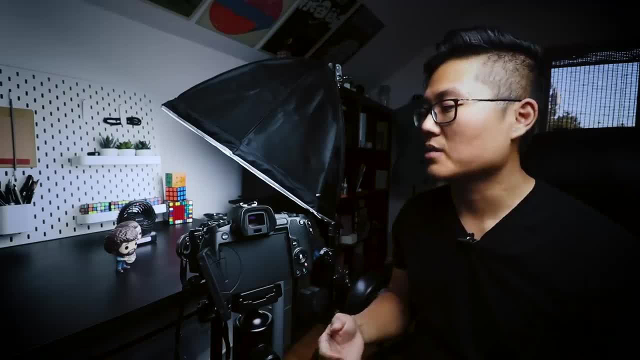 fine-tuned, So you want to keep your aperture small so that everyone's fine-tuned, So you want- is in focus, but then that underexposes everything. so you have to slow down your shutter speed, but then, because the children are moving, you want to increase the shutter speed. whenever i'm taking 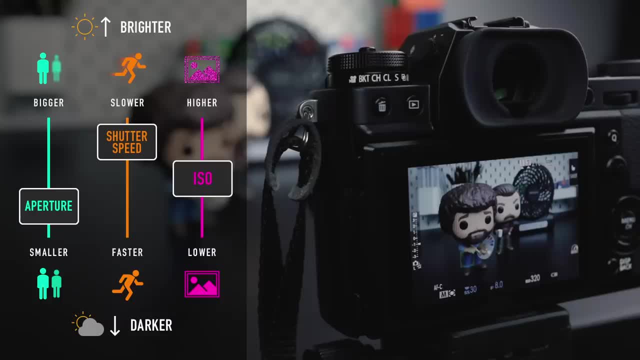 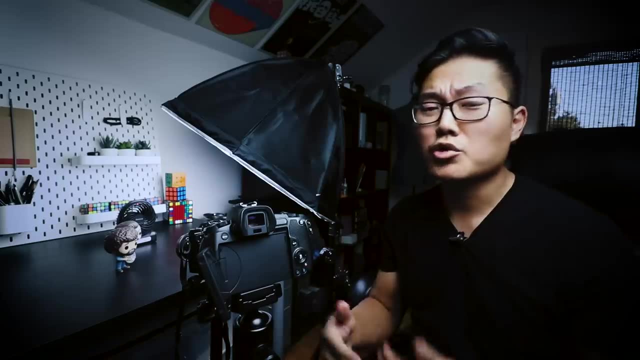 pictures of people or anything alive. i usually keep my shutter speed above 1 25th of the second, or sometimes 250 or 500, just to be safe, and when you're shooting in the sun or when you're shooting with flash, you can obviously go higher than that. but now we have to work with what we've got right. 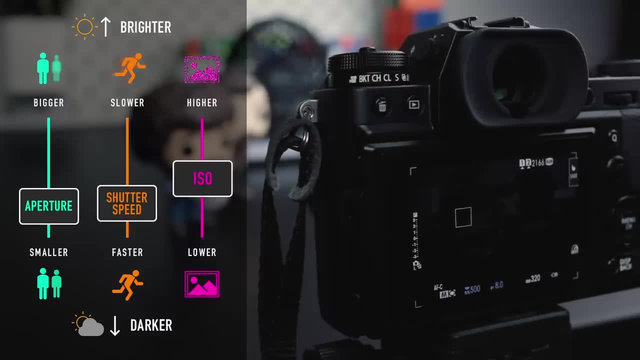 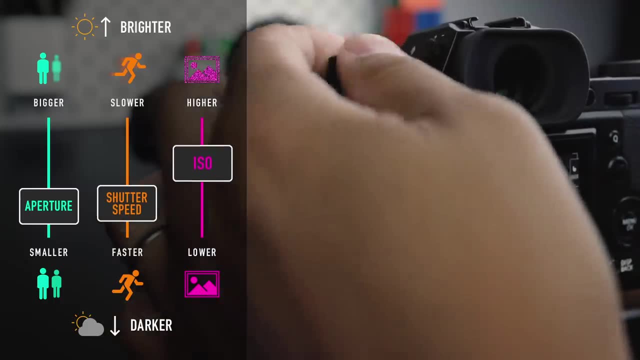 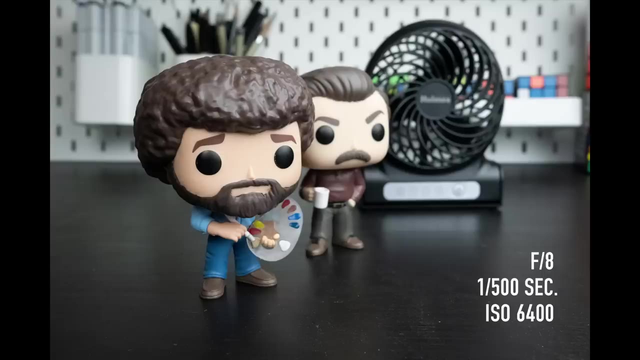 now i'm at f8 and 1 500th of the second and, as you can see, everything is clearly underexposed. so what do you do now? now is the time you can increase your iso and now, as you can see, i'm at iso 6400 and, as you can see, everything is nicely exposed, everyone is in focus and the shutter speed. 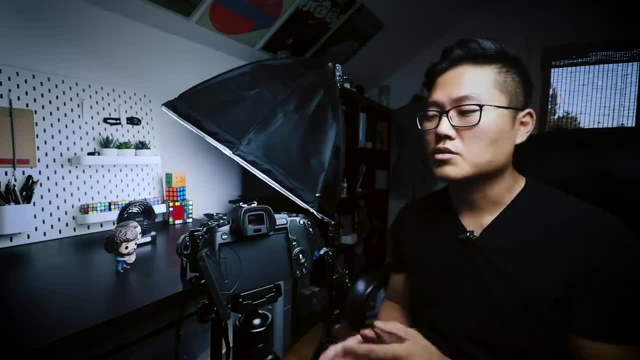 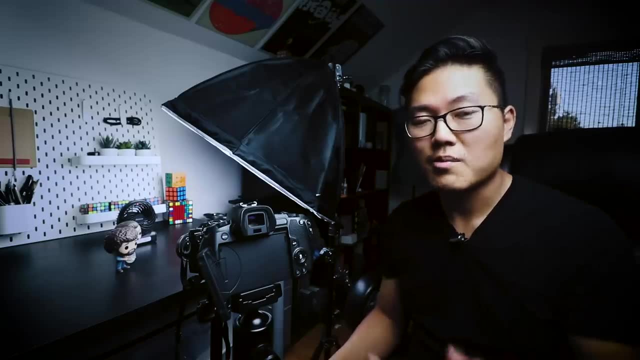 was quick enough to freeze the movement. but using high iso also has its own side effects. remember when i said that iso is like a volume knob on a stereo or a microphone. what happens when you increase the volume to the max? you start to get nasty feedback and your sound gets all. 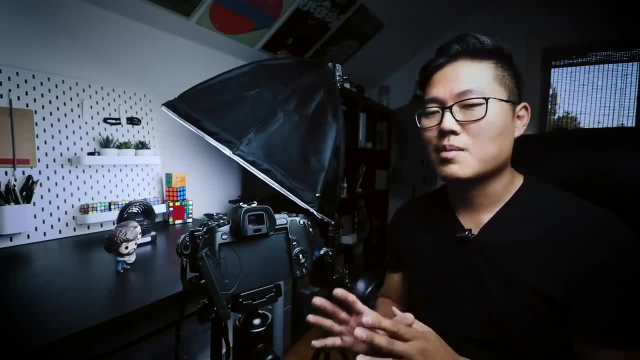 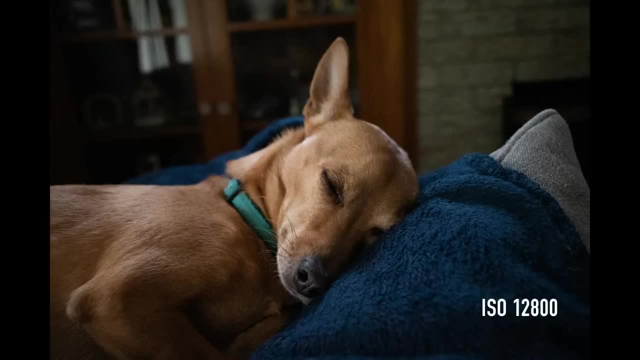 distorted and it doesn't sound very good. the similar thing happens when you increase the iso too much on your camera. so when you increase the sensitivity of your camera too much, it starts to pick up all kinds of noise and grain in your photos and your pictures come out all purple. 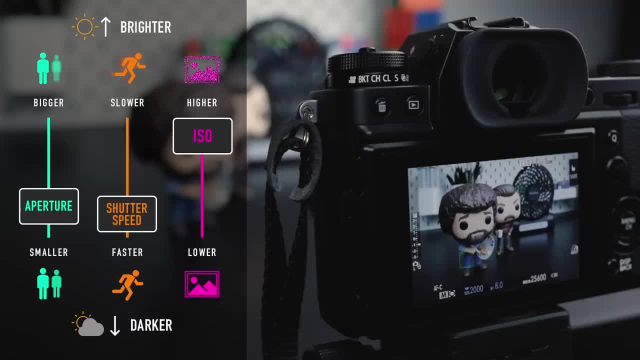 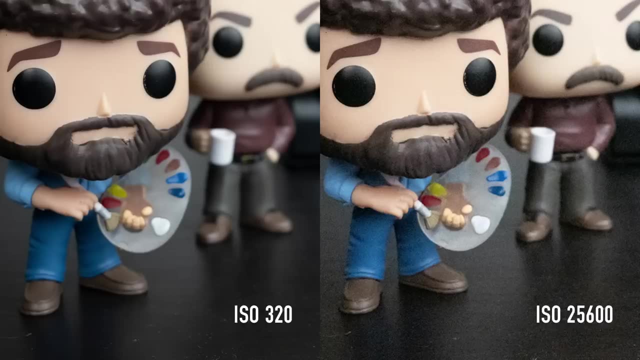 and green and smudgy and it just doesn't look very good. and just to kind of demonstrate that, i'm going to take a photo at iso 25 600 and you'll be able to see the clear picture difference. so whenever possible you want to keep your iso as low as possible to get the best results. 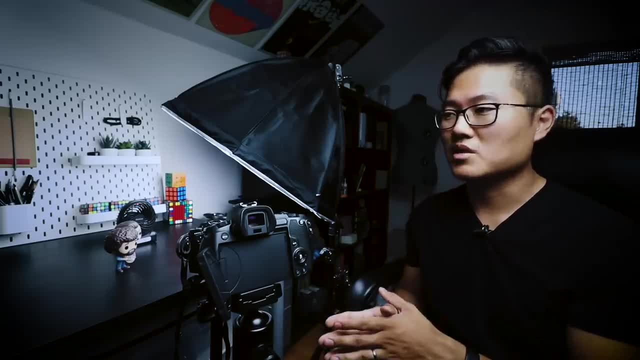 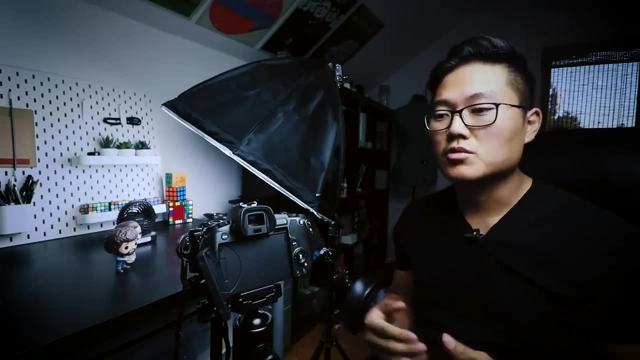 the differences might be subtle, but you can still tell the difference between iso 100 and 200 and 200 and 400, and it just gets worse and worse as you go higher. so, depending on what you're trying to do, you always want to start with either aperture or shutter speed and then adjust the iso only when 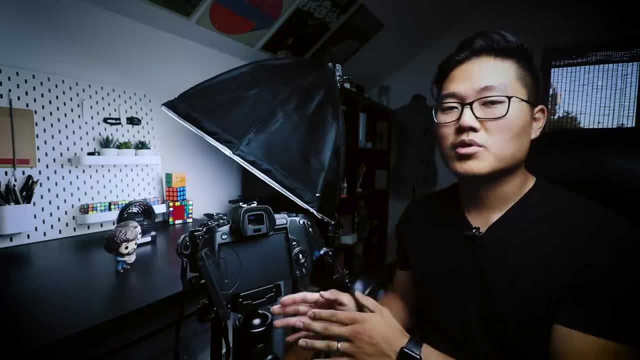 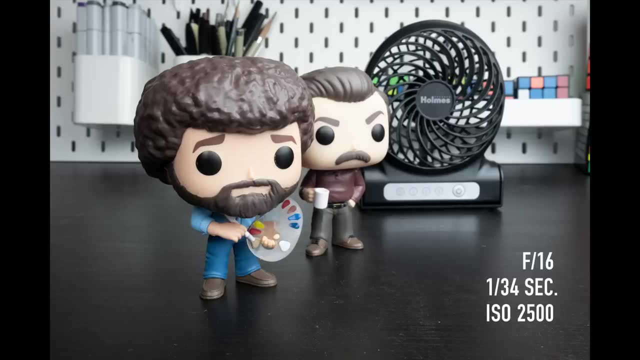 you need to. so now that you understand what these are, i'm going to put everything into auto and see what the camera does. so, with that photo, the camera decided to take the photo at f16, at 1: 34th of the second- which is kind of odd- and iso 2500. so that's what the camera decided to do in full auto. 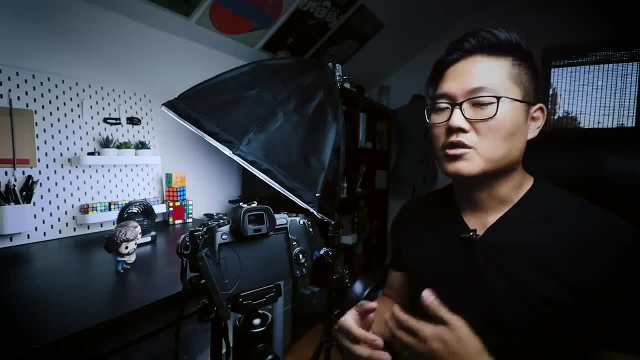 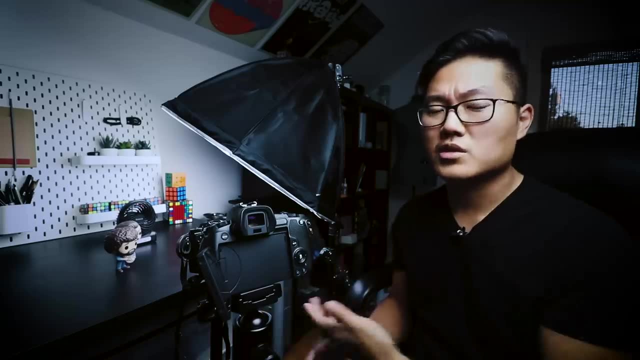 so the problem here is, no matter how expensive it is or no matter how good it is, your camera is not very smart. it's not going to be able to read your mind on what you're trying to do, so it does not know that. if i wanted to take a portrait of bob ross, 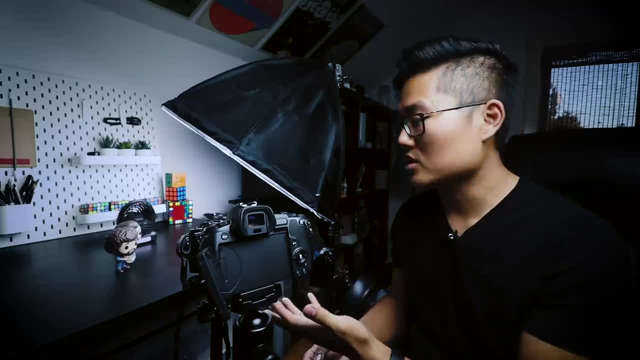 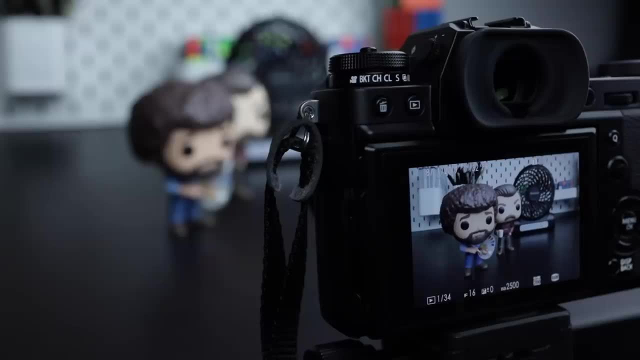 with blurry background, or if i wanted to keep the iso as low as possible, or if i wanted faster shutter speed to freeze the movement, it does not know. i just simply press the shutter button and it did what it thought was the best for the situation. so that's what really shooting manual does for you. 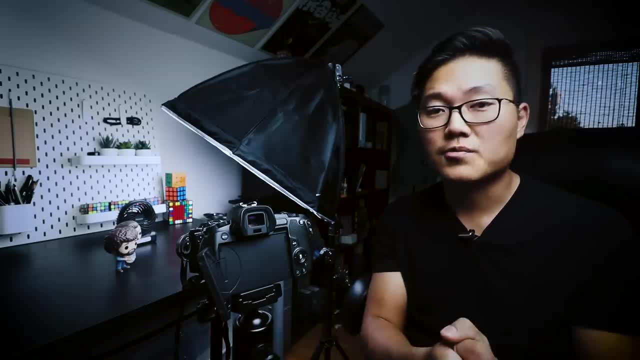 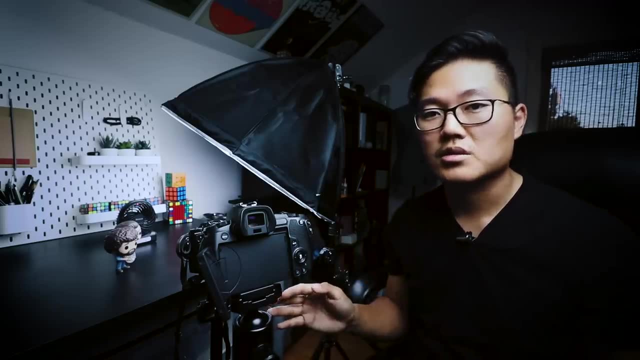 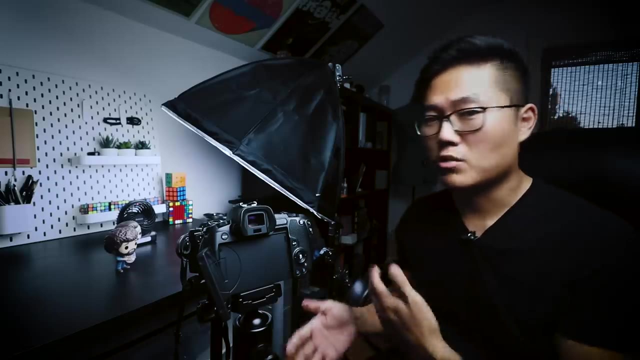 and your photography shooting manual gives you, the photographer, the full control, so you can take your camera's ability to its full potential in any situations. that way, if i want to take a portrait of bob ross with a nice blurry background, I can do that if I want both Bob Ross and Ron Swanson to be in focus. 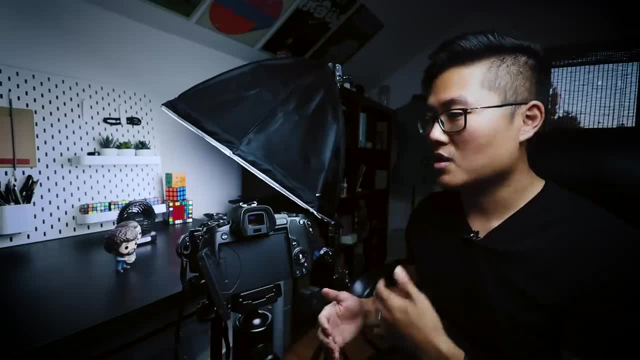 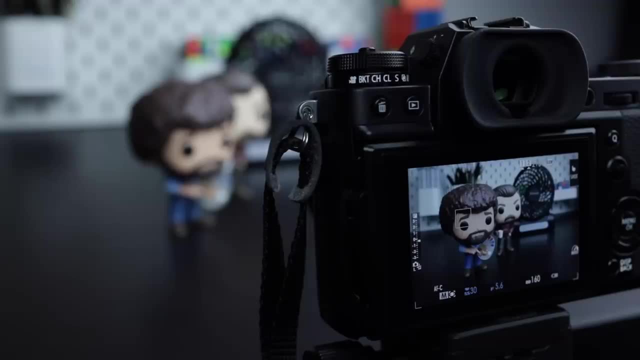 I can make the aperture smaller and slow down my shutter speed to compensate the lack of exposure. And if I want to increase the shutter speed, for whatever reason, I can either make the aperture bigger again or increase my ISO. So that's how you shoot manual. 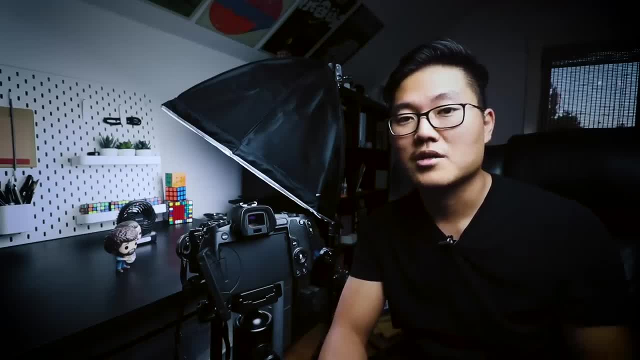 And please feel free to leave me any comments or questions, if you have any, And I'll show you, guys, some more examples of photos that were taken at different settings. So take a look, And that's it for me today, And thank you for watching, as always. 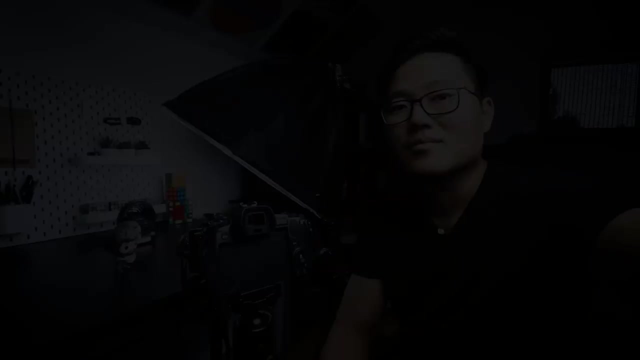 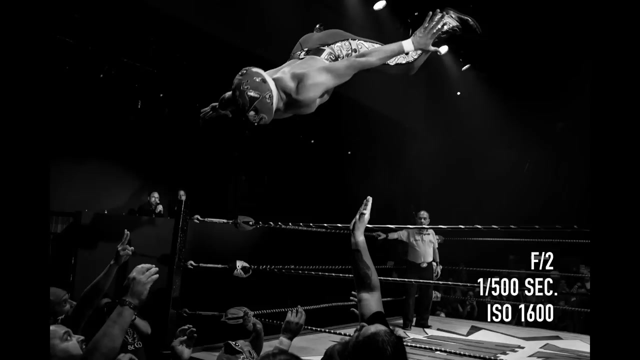 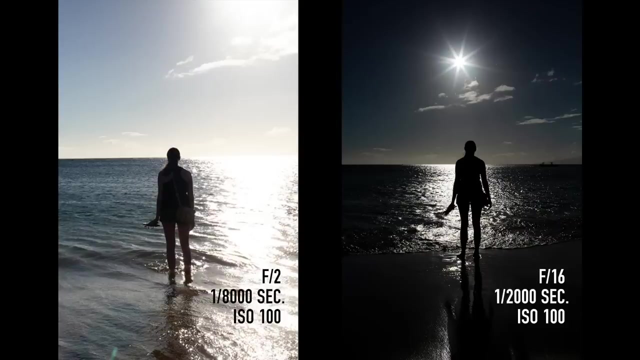 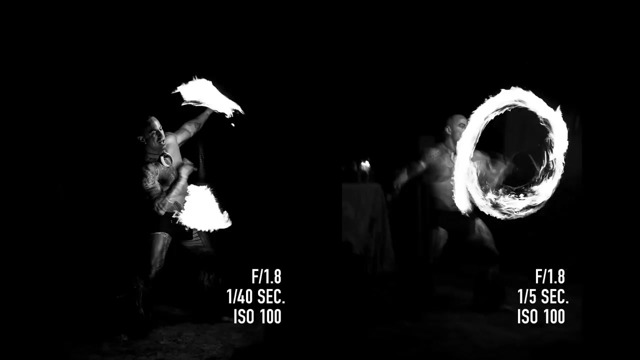 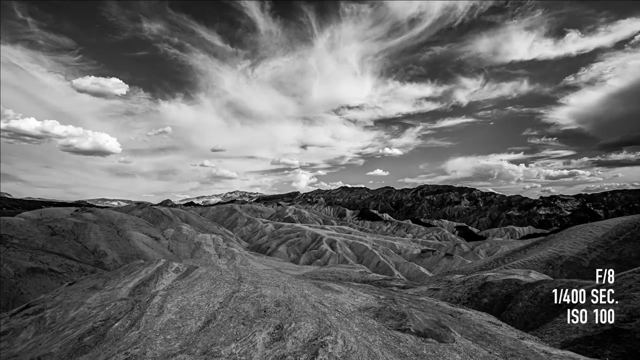 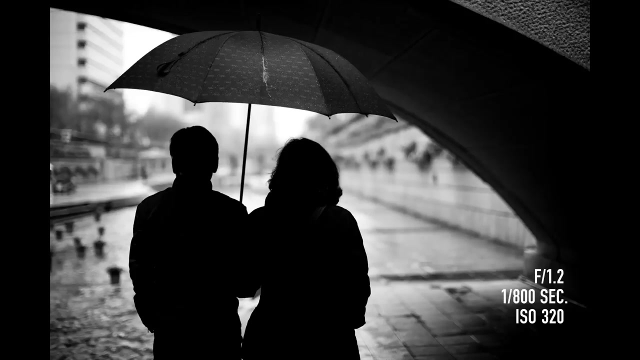 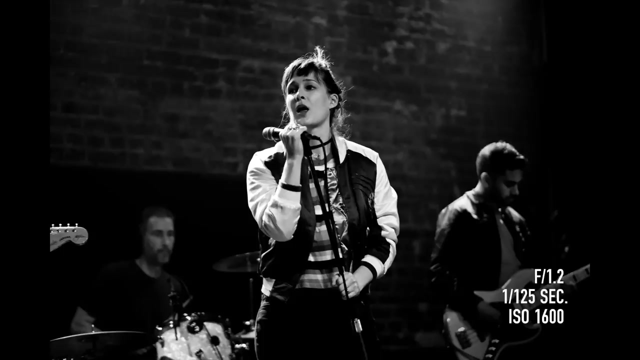 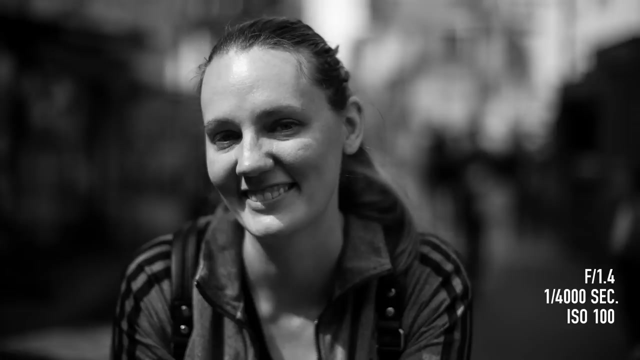 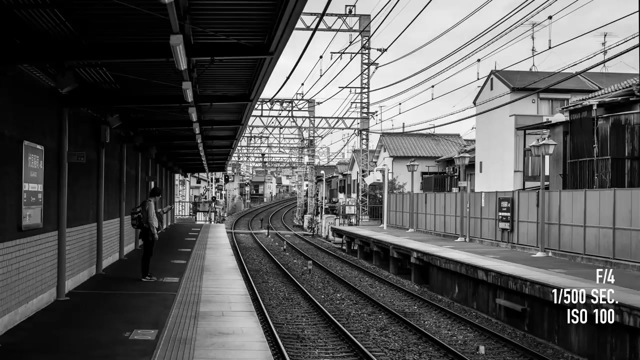 And I'll see you next time. Bye-bye. 🎵, 🎵, 🎵, 🎵, 🎵 🎵. Thank you.